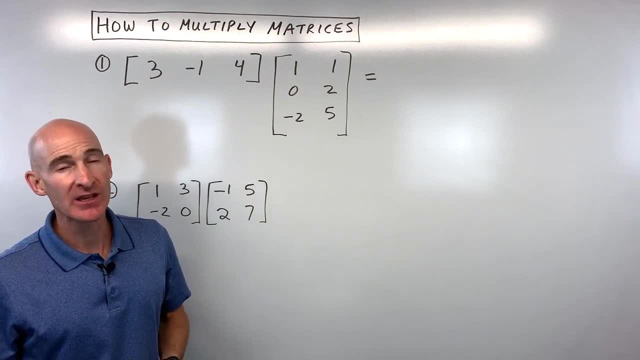 In this video you're going to learn how to multiply matrices. so we're going to go through four examples together. I'm going to show you how to do this. Let's dive in The first example. here we've got this matrix times, this matrix. Now, first of all, you might be saying what's a matrix? Well, it's just a. 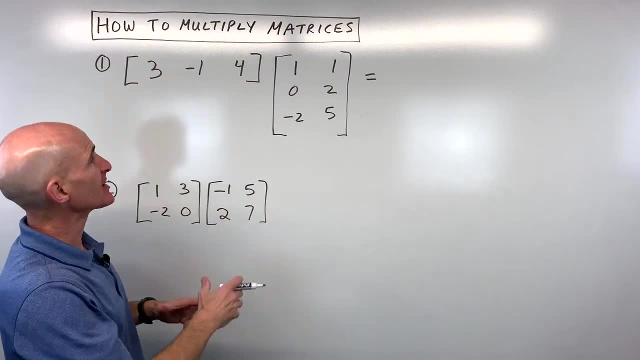 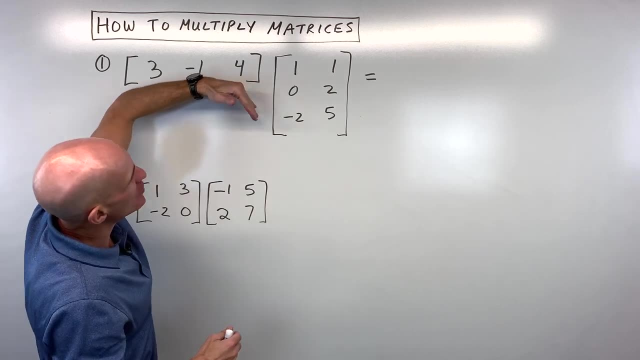 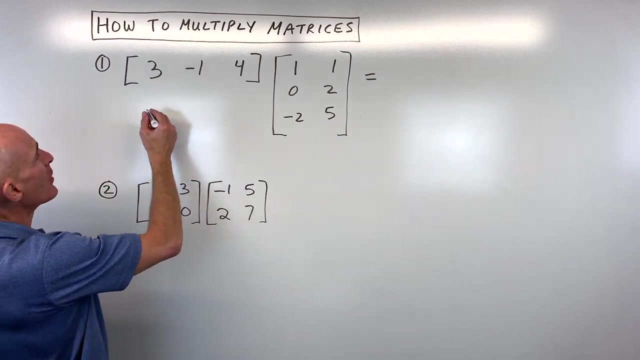 way of organizing data. Okay, it's almost like a table or a chart, and what's interesting is that when you multiply matrices, you're multiplying these quantities together and you have to make sure that the dimensions match up. So what do I mean by the dimensions? Well, you want to always. 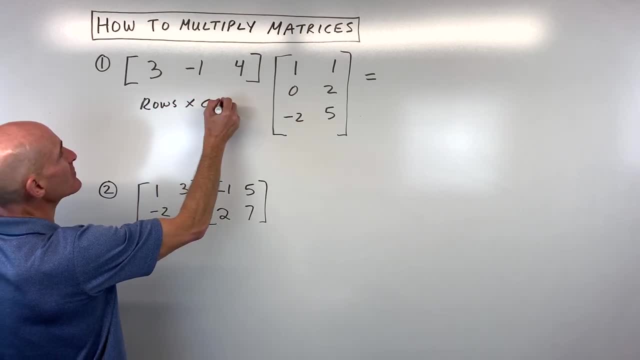 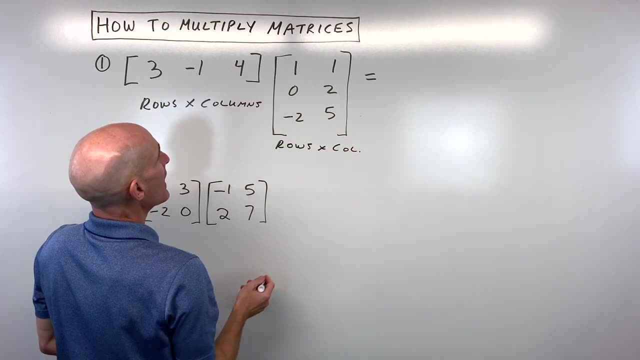 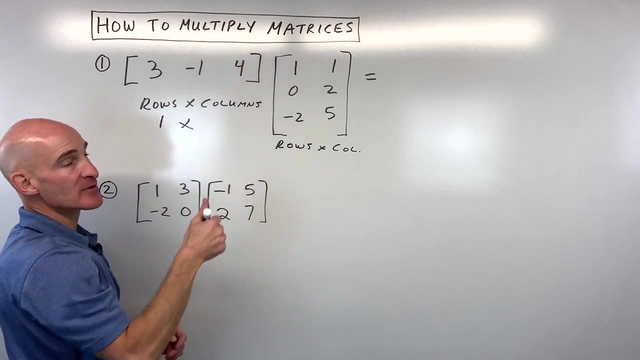 figure out what the rows are by the columns. Okay, and the same thing with this matrix. You want the number of rows by the number of columns, And so the rows go this way. Okay, so we can see that there's one row here and the columns go like Roman columns, like in the vertical direction. 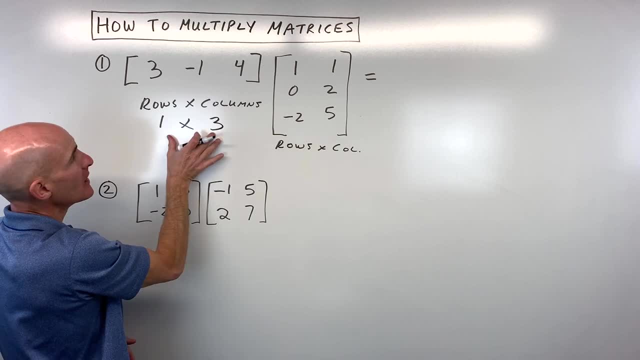 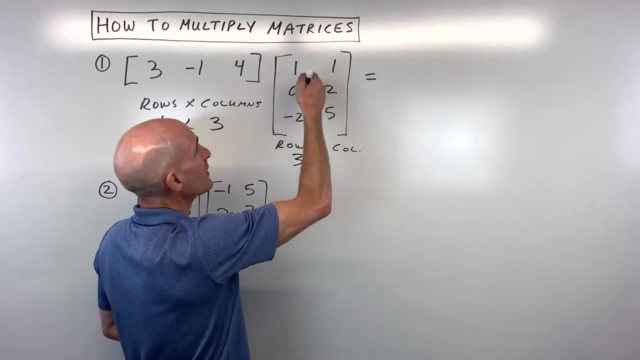 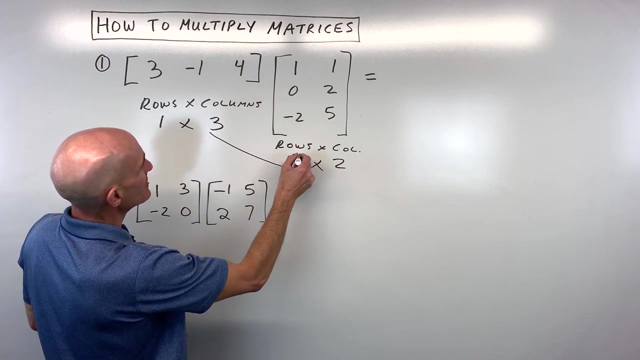 So you can see one, two, three. So we have a one by three matrix here, and over here we'll have, let's see, one, two, three rows and we have one, two columns. So when you multiply matrices you want to make sure that these inner dimensions they're the same, that they match, And you're. 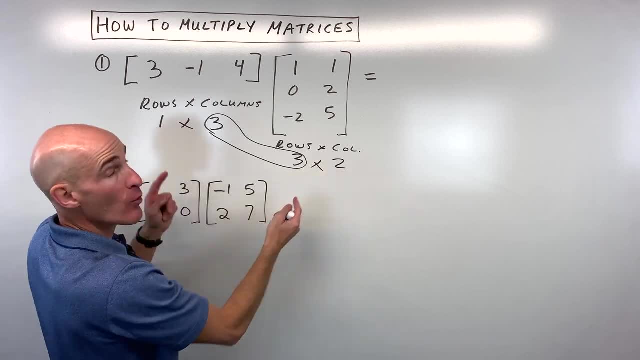 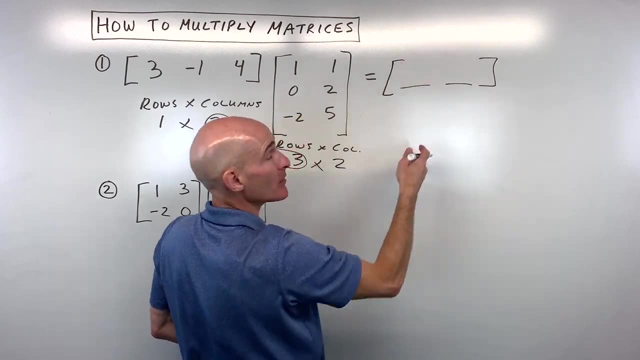 going to end up with a matrix that has these outer dimensions. It's going to be a one by two. So what that means is we're going to have one row and two columns. Now, remember always rows first and columns second. So rows by columns, rows by. 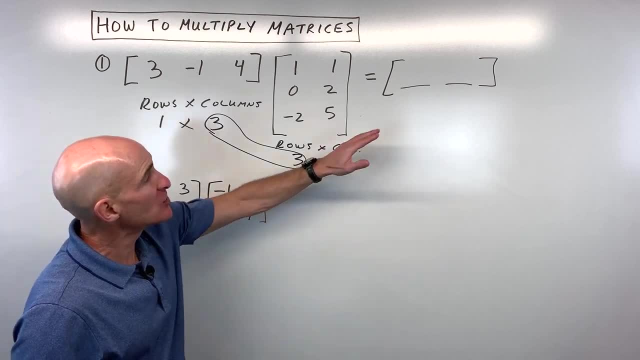 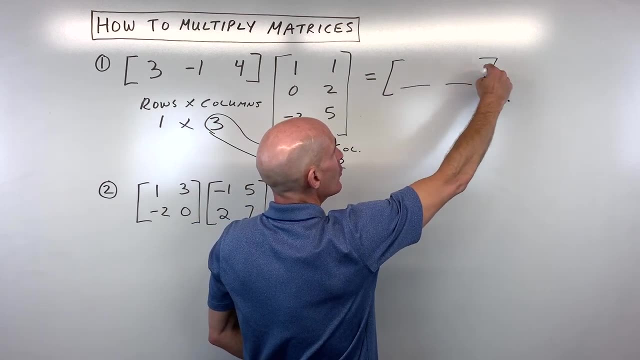 columns forever and ever. Okay, so now, what I like to do is I like to work backwards a little bit. I like to say: what position is this element in? Well, this element is in the first row, first column. So that tells me what to do. I'm going to take this first row here. 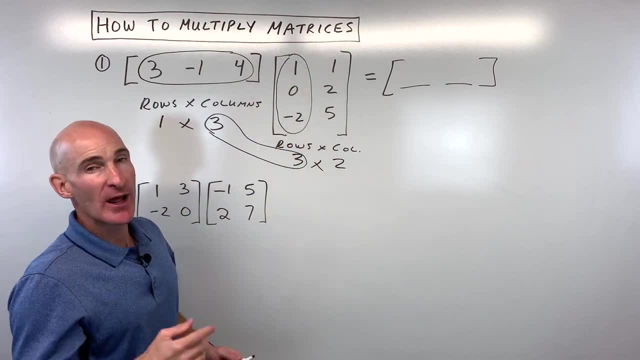 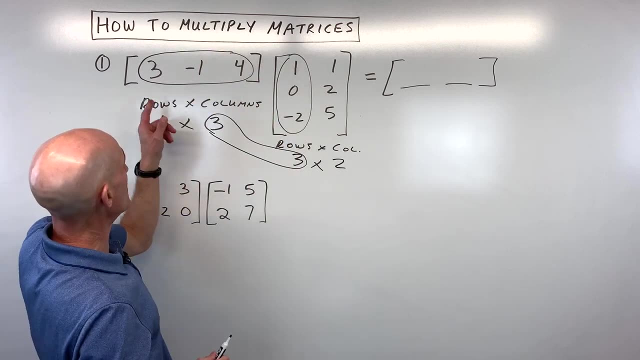 I'm going to multiply it by this first column here, But what I do in my mind is I take this row and I rotate it so that the elements match up with each other. So what I mean by that is I take the first element in this row times the first element in this column and I multiply them together, So I 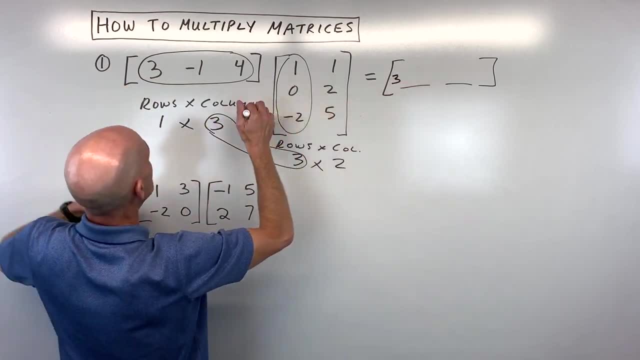 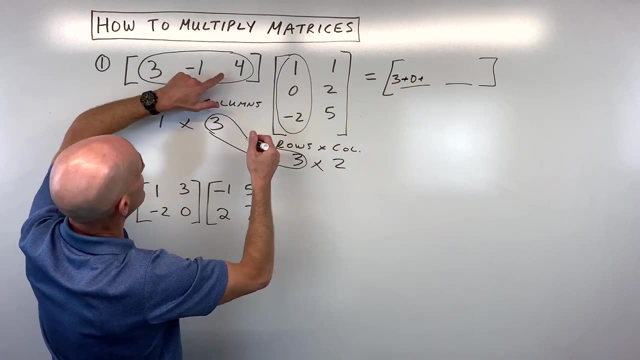 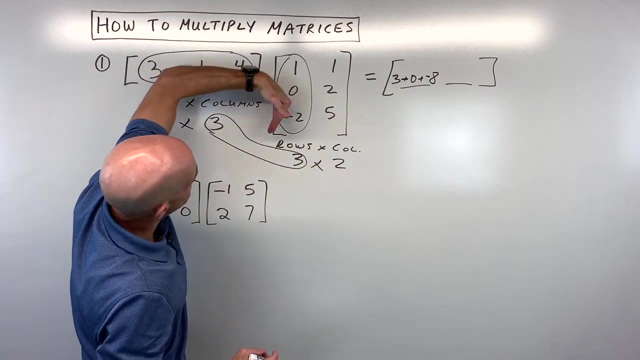 say three times one is three. Then I take the second element, second element, So negative one times zero is zero. And then I take the third element and the third element, So four times negative two is negative eight. And so you can see that we multiply these ones that match up with. 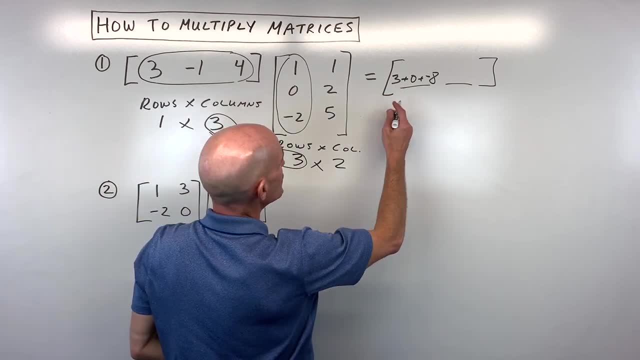 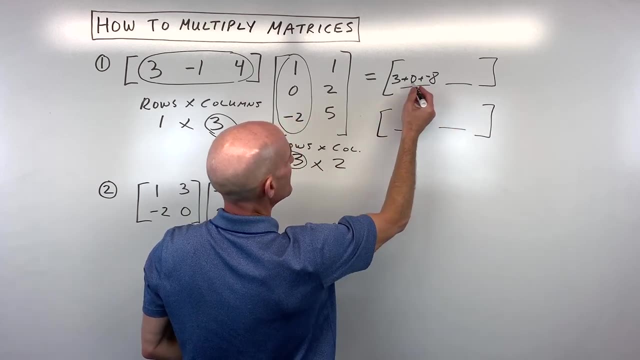 each other and then we add those quantities together. So sometimes I'll just make kind of like a little matrix Here and then I'll put the final result like in another matrix, just so I can do my calculations. So three plus zero plus negative eight is going to be negative five. Now this one. 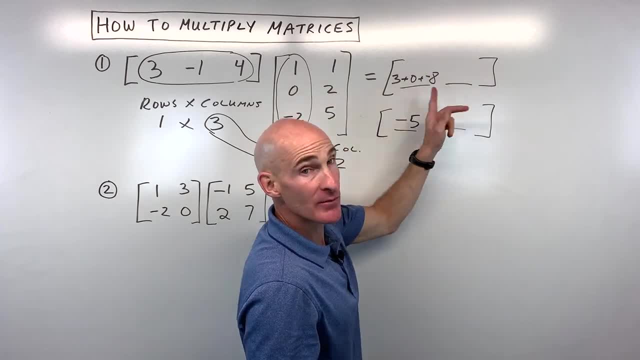 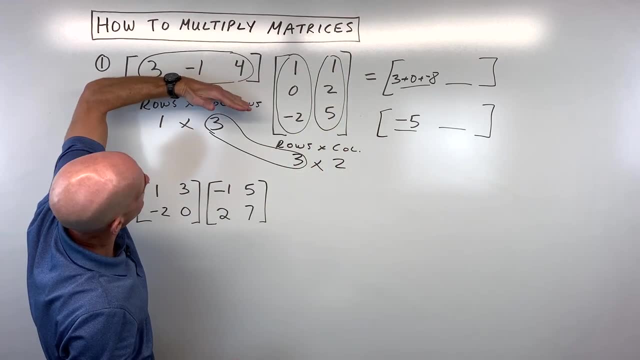 is in the first row, second column. So that tells us what to do. We're going to take this first row times, this second column. Now you can either do my technique of taking this row and kind of rotating it- Okay, like that- Or you can just say first and first, second and second. 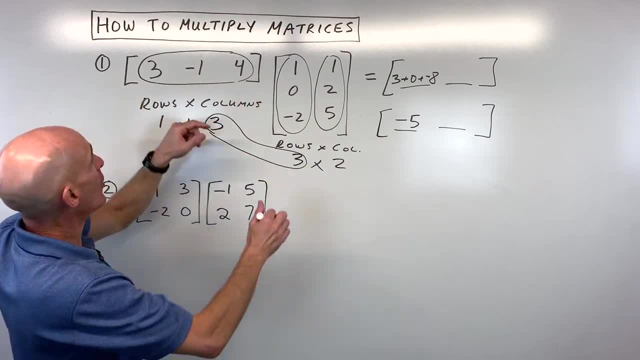 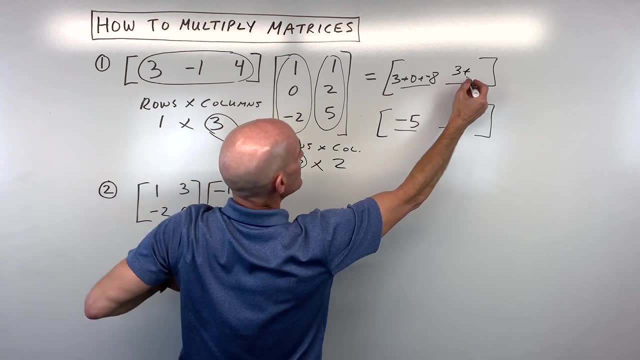 third and third, You're going to multiply those and then add them together, So let's do that. So two times one is three. Some people are good at doing this in their head. I like to write it down: Negative one times two is negative two, And then four times five is twenty. If we add all those, 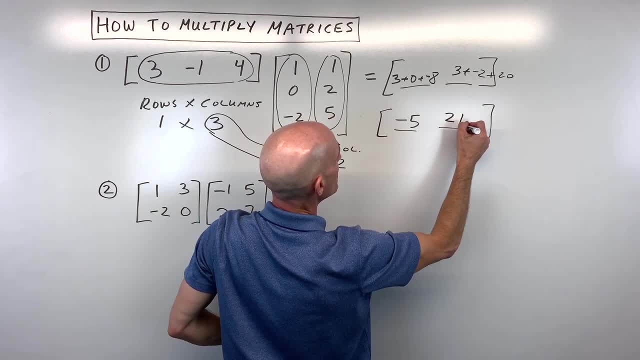 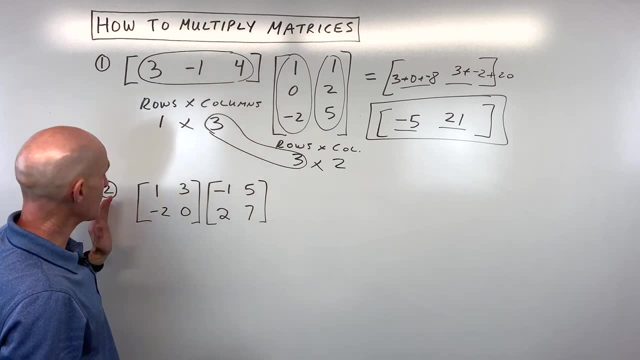 together. let's see what we get. This comes out to: one plus twenty is twenty-one, And this is our final result. Okay, let's take a look at another example For number two. what are the dimensions of these two matrices? Well, let's see, We've got one, two rows, Remember? the rows go this: 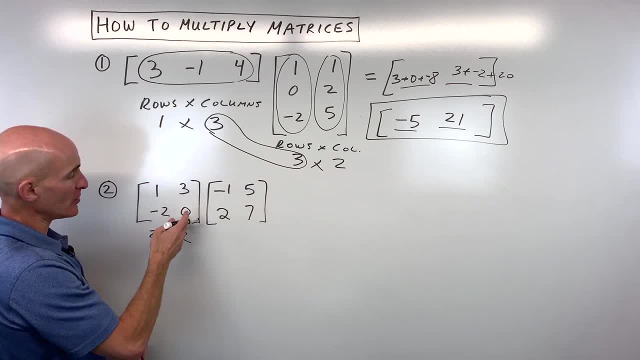 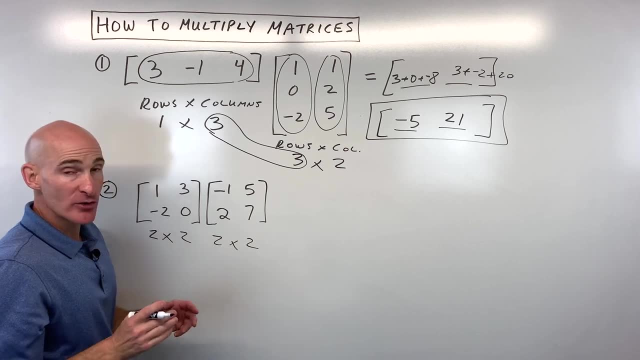 and we have one, two Roman columns. right, They go vertically. Same thing with this one. We have one, two rows and one, two columns. Remember, always, rows first, columns second, forever and ever. Okay, now we call these square matrices because you can see, it's like a square, The same number of rows. 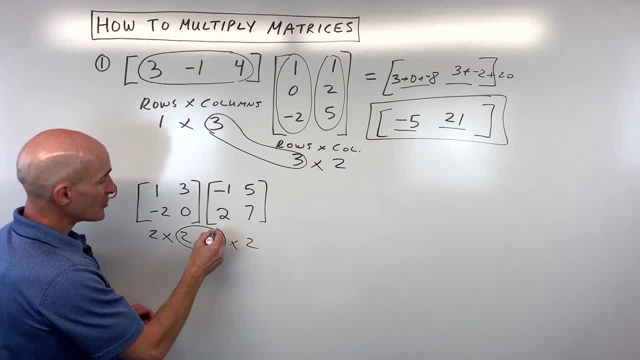 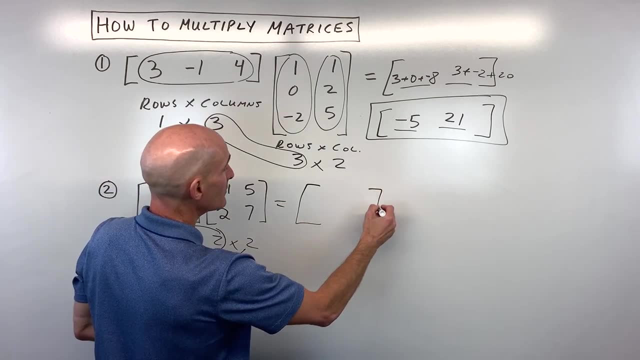 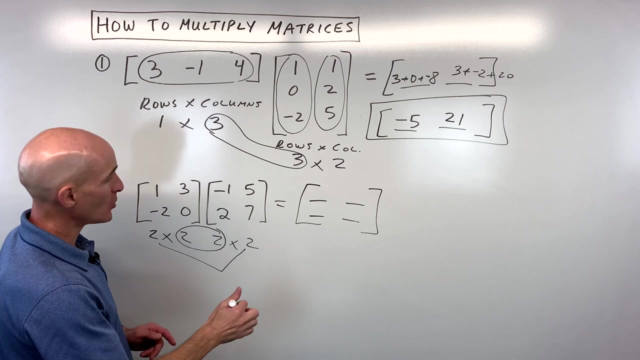 and columns. Okay, it looks like a square. You want to make sure that the inner dimensions match, which they do, And you end up with a matrix that has these outer dimensions. It's going to be a two row, two column matrix. So one, two rows, two columns- Okay. so now let's do our calculations So you can do them in. 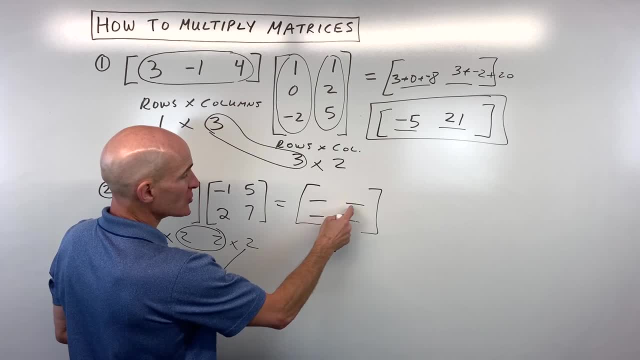 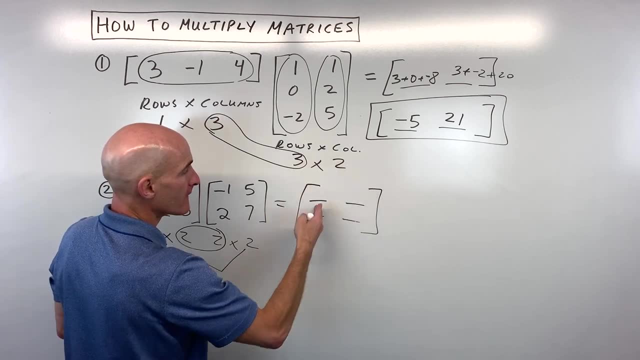 any order you want, Like you could start with this one or this one, or you can do them in any order. It doesn't matter. But what I like to do is kind of work backwards. I like to say: what position is this in? It's in the first row, first column. Remember, rows first, columns second. So that tells. 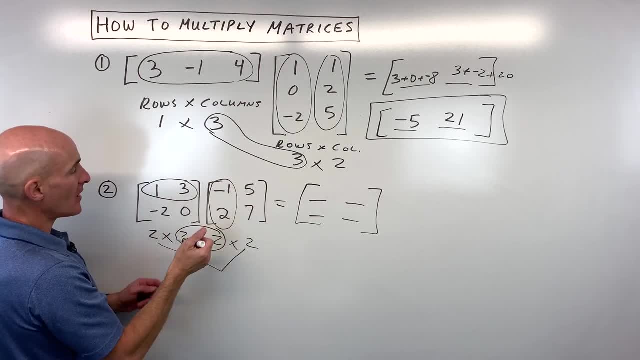 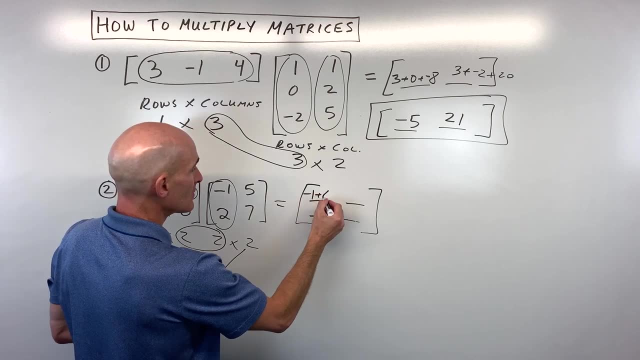 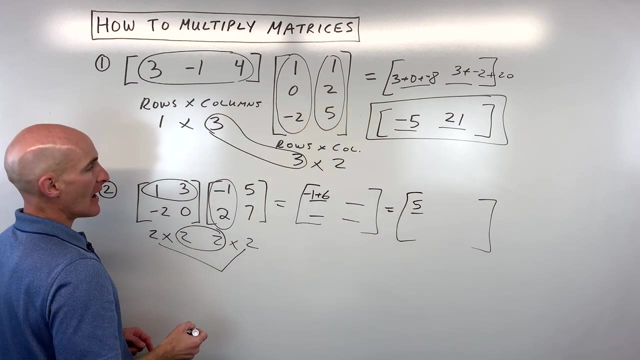 me what to do. I'm going to take the first row. times the first column One times negative. one is negative one. The second one is negative one. Three times two is six. Add those together, put it in the final matrix over here, which is five. Okay, now let's go to this one here. This is in what position? The first row. 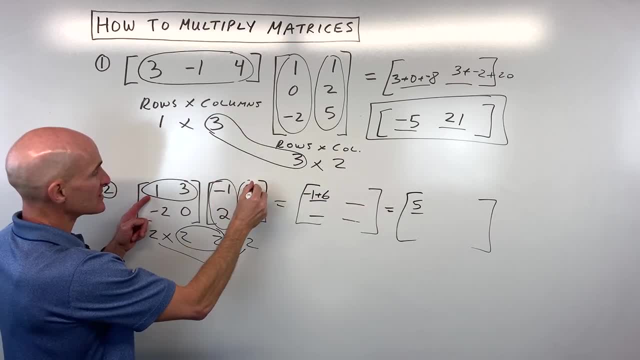 second column: right? So that tells us what to do. First row times, second column: You can either do my technique of rotating and multiplying the ones that match up, Or you can do first and first, second and second and then add them together. One times five is five plus. 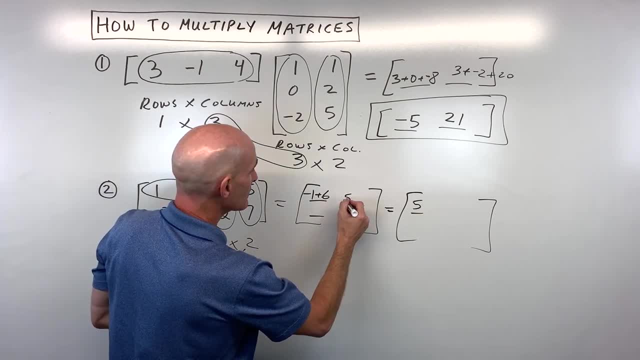 You can either do my technique of rotating and multiplying the ones that match up, or you can do first and first, second and second and then add them together. One times five is five plus 5 is 5, plus 3 times 7 is 21.. 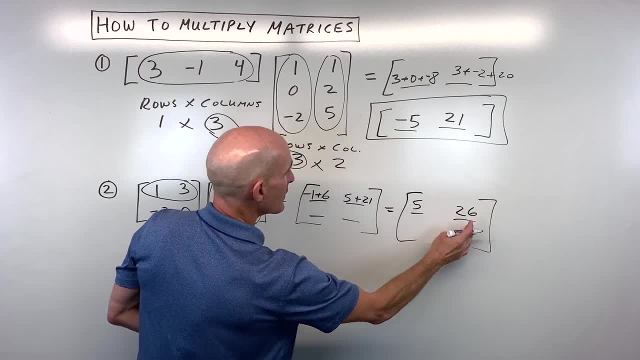 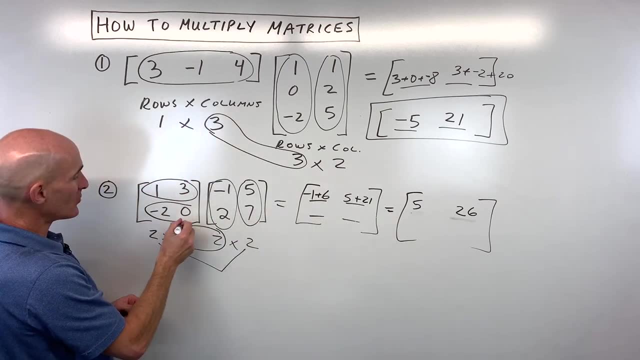 Add those guys together: 26.. You don't have to put these lines here, I was just kind of doing that. Okay, now this one. we've got the second row, first column. So that tells us what to do. Second row times, the first column. 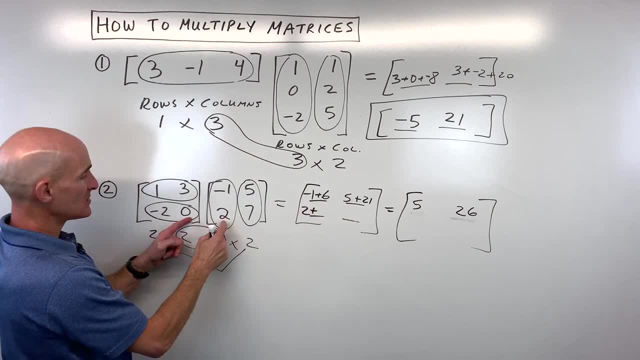 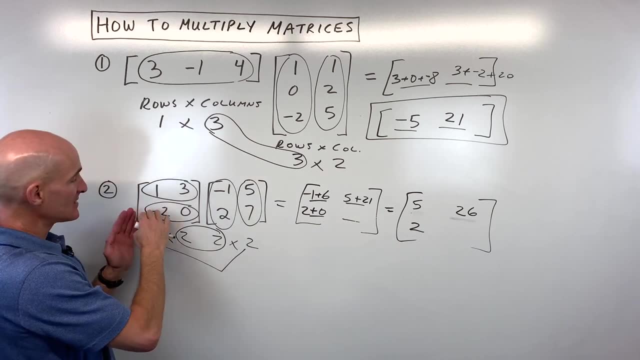 Negative. 2 times negative, 1 is 2, plus 0 times 2 is 0.. 2 plus 0 is 2.. Last one, second row, second column. Second row, second column. So we have negative 10 plus 0, which is negative 10.. 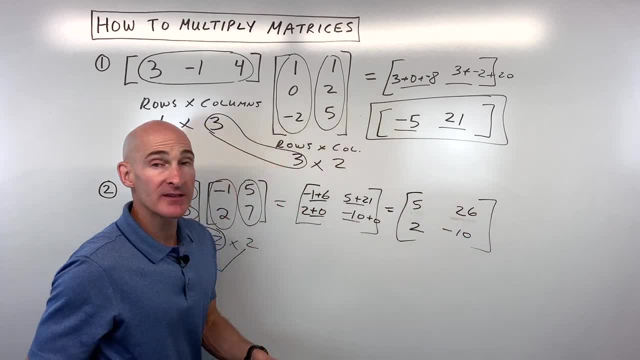 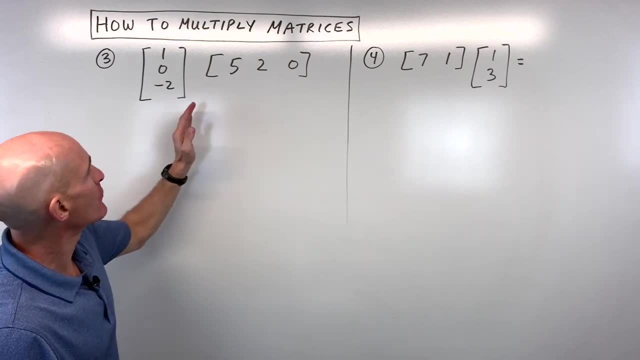 And this is your final result. Let's take a look at two more examples. Okay, if you're getting the hang of this, try number 3 and 4 on your own. We'll go through them together. I want to make a couple other points to you while we go through these. 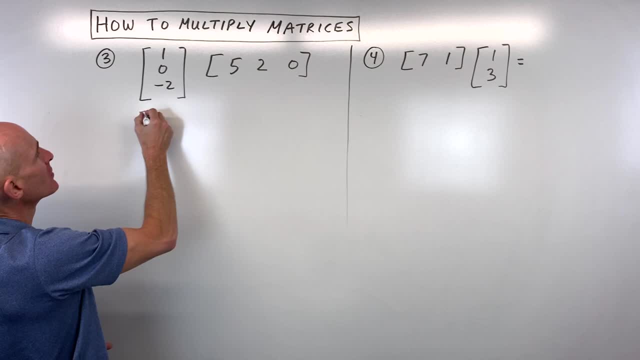 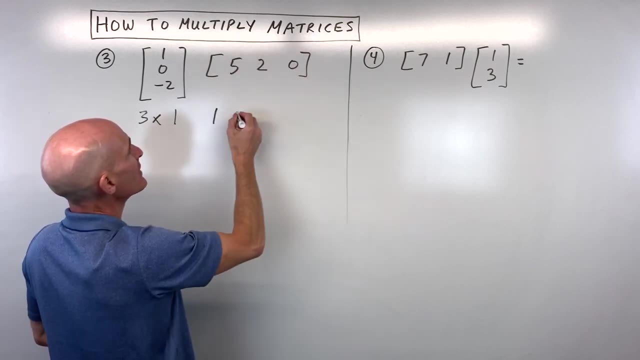 Notice this matrix- here is a 1,, 2, 3 rows by 1 column, whereas this matrix is a 1 row by 1,, 2, 3 columns- And notice that these inner dimensions they match. but you might be saying, Mario, what happens if they don't match? 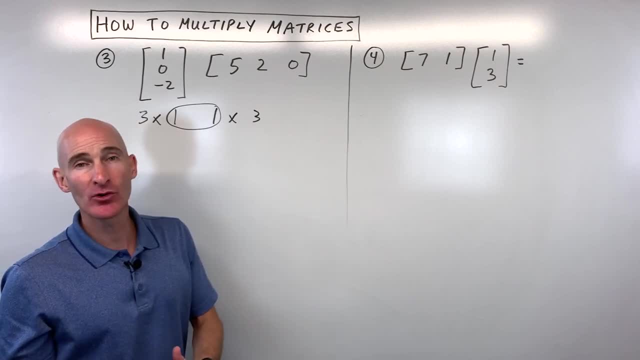 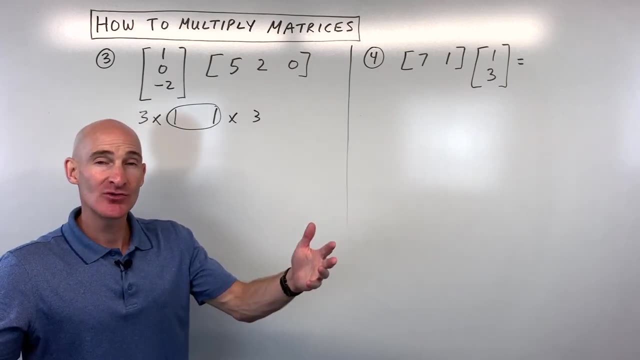 Well then it just means it's a dimensional mismatch or it's just not possible to multiply the matrices together. You're not going to be able to do it. The other thing that's interesting is that in normal multiplication, 5 times 2 is the same as 2 times 5.. 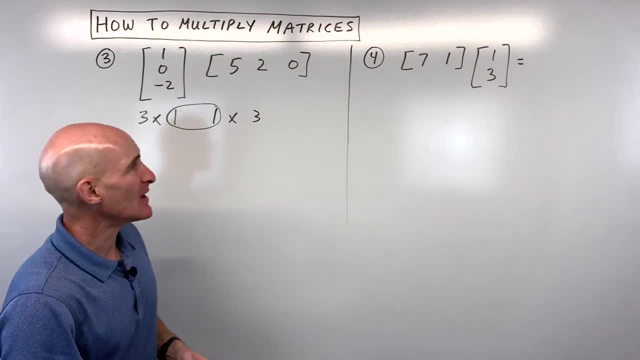 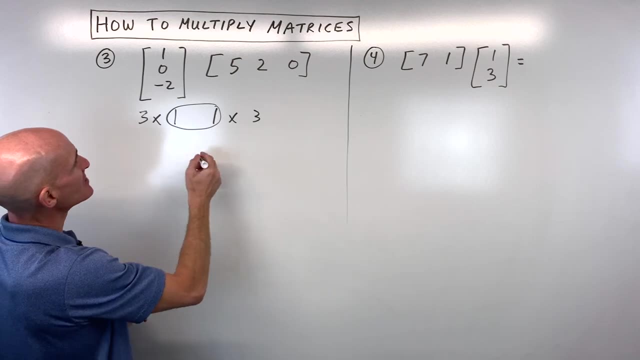 It doesn't matter the order right, It's commutative right. But with matrices not necessarily commutative, because if I were to take this matrix and put it here, what we would have is we would have a 1 by 3 and then by a 3 by 1,. 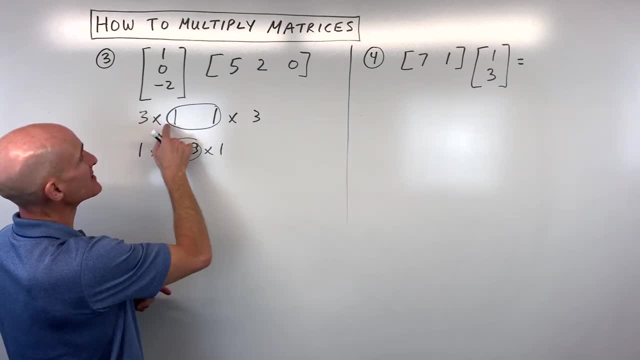 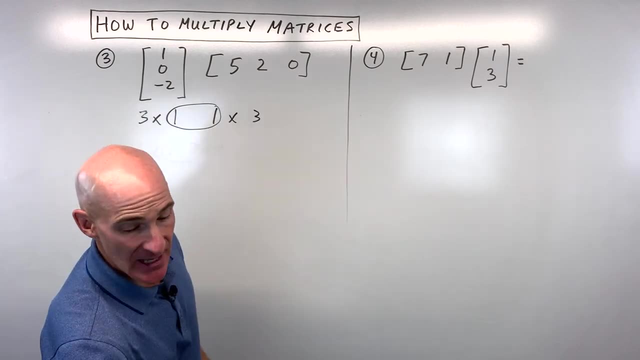 the dimensions are matching, which is great, but we're ending up with a 1 by 1 instead of a 3 by 3.. It's a completely different size matrix, So they're obviously not going to be the same, which means that multiplication with matrices is not commutative, right? 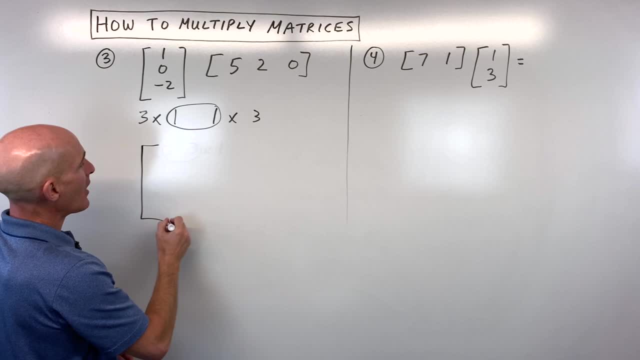 But for this one we're going to end up with a 3 by 3.. So let's see if we can draw that out. So a 3 by 3 means we have 3 rows and 3 columns. So 1, 2, 3 rows, 1, 2, 3 columns. 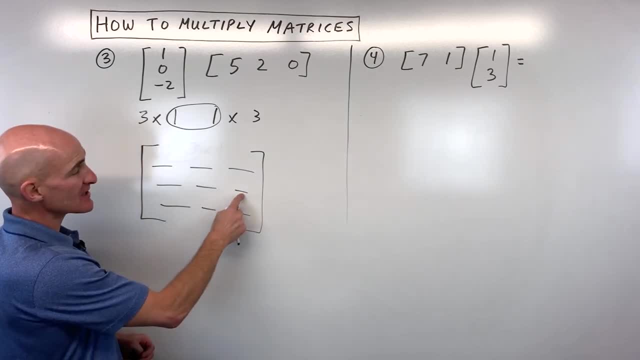 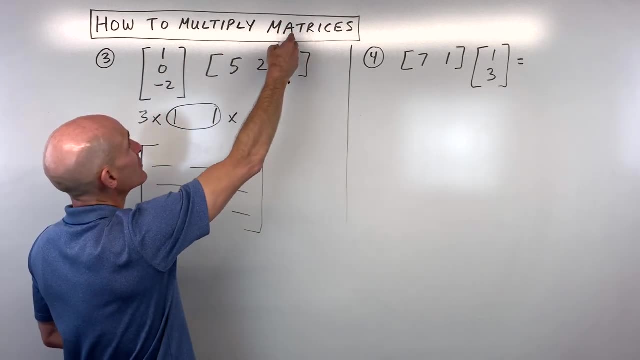 And again, remember how I said: you can do this in any order, Like if I wanted to find just this element here, I say that's in the second row, third column. So I take the second row, which is 0, times the third column, which is 0, that's going to be 0.. 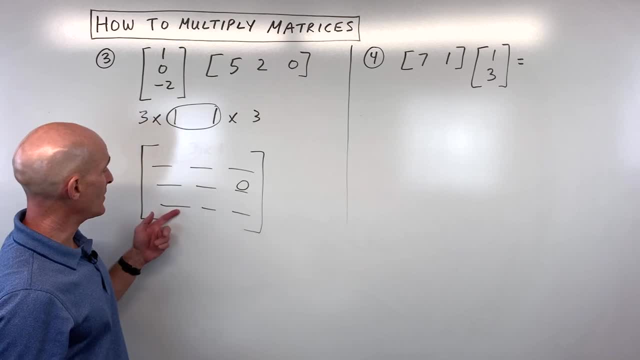 See, Sometimes you don't need to figure out the whole matrix, You just need one element. Say: if I want this one, third row, first column, third row, first column- So negative 2 times 5 is negative 10.. 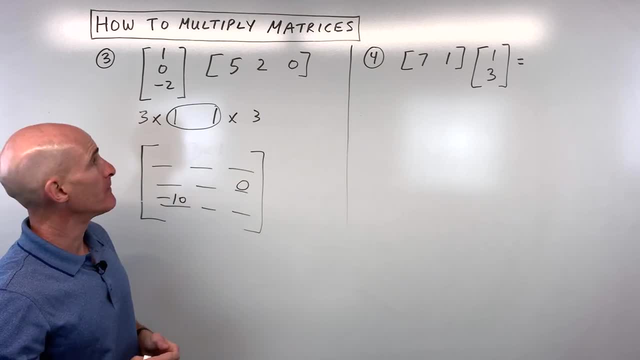 Now this is interesting. There's nothing to add in this particular problem because you just have one element in the row, one element in the column. Let's say, we want to do this one right here. This is in the first row, second column. 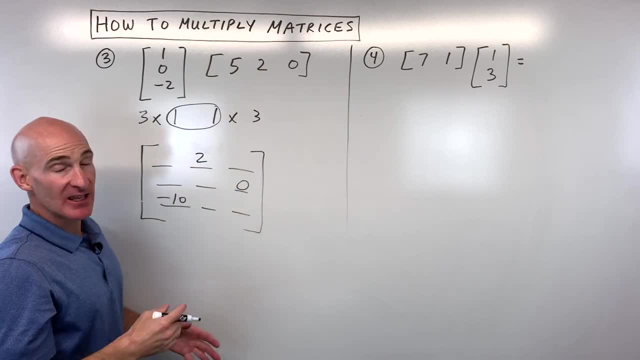 So first row, second column. Now that's kind of chaotic, right, You're just jumping all around. But if you have to do the whole thing, I kind of work from left to right, from top to bottom, like that. So I would start here. 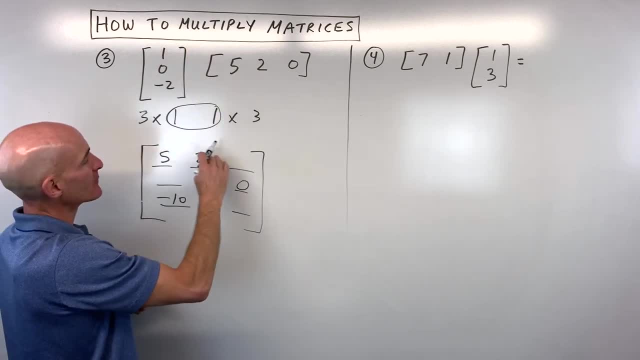 First row, first column, that's going to be 5.. First row, third column, that's going to be 0.. This one is in the second row, first column. So 0 times 5 is 0.. And this one's second row, second column, which is 0.. 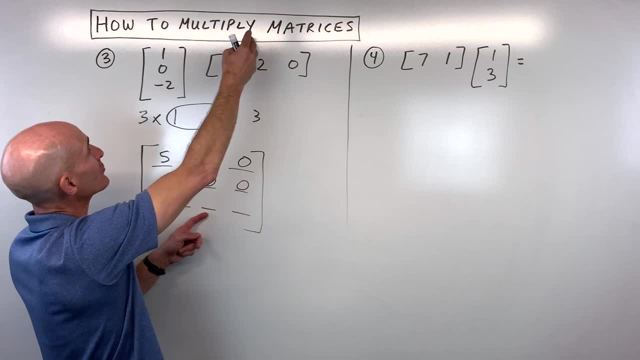 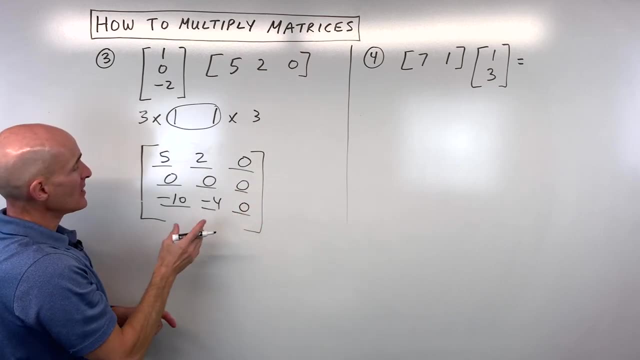 And then over here we've got a third row, second column. So third row, second column, that's negative, 4.. And over here we have third row, third column, which is 0.. So that's our final resultant matrix. 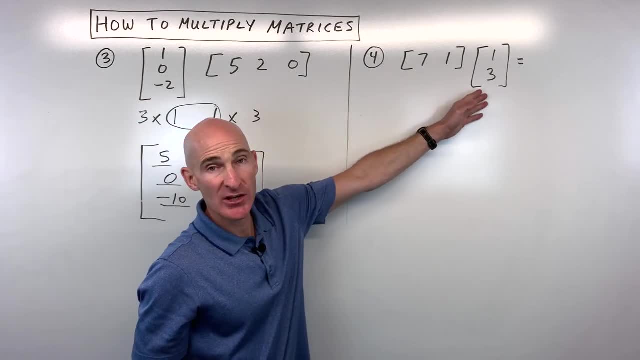 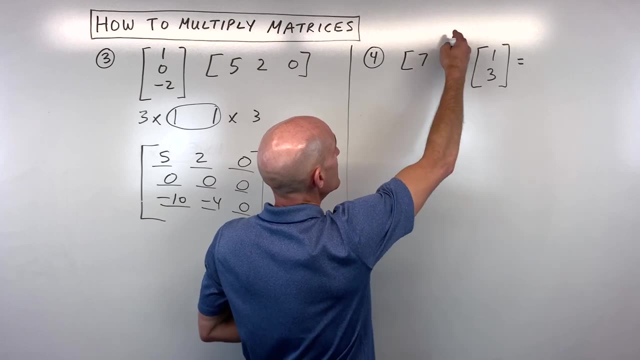 Okay for number 4,. why don't you try this one if you can? What are the dimensions? Do they match up And how would you multiply them together? Well, let's see. If I was going to do it, I can see. I have one row, two columns.